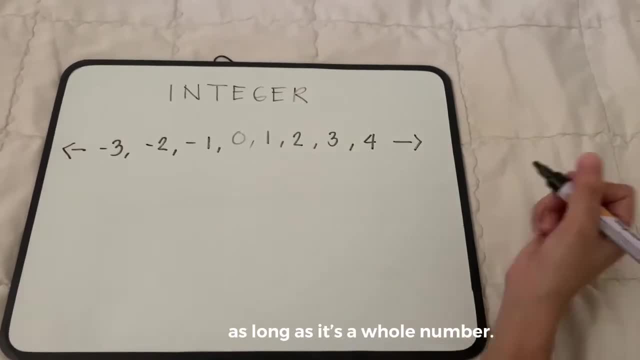 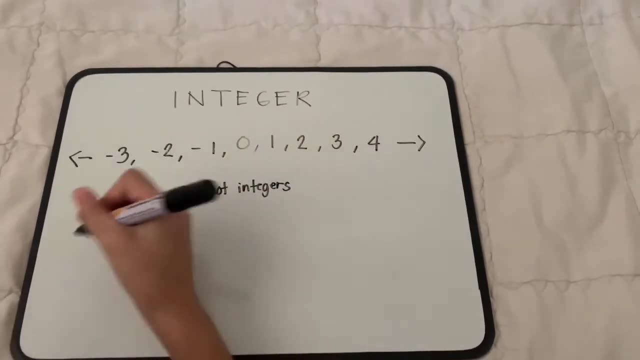 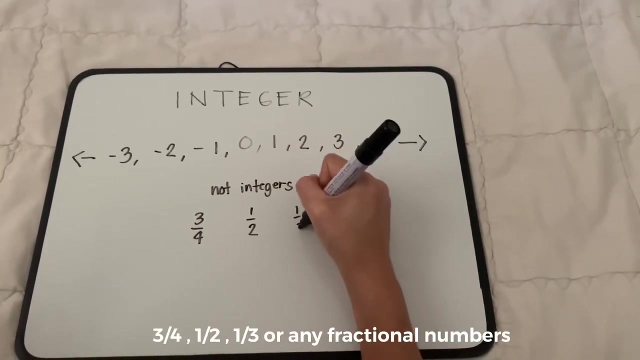 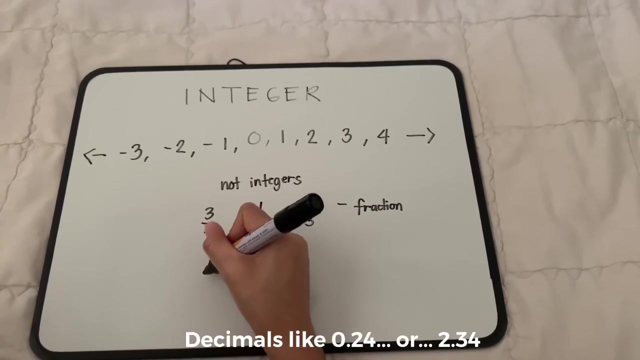 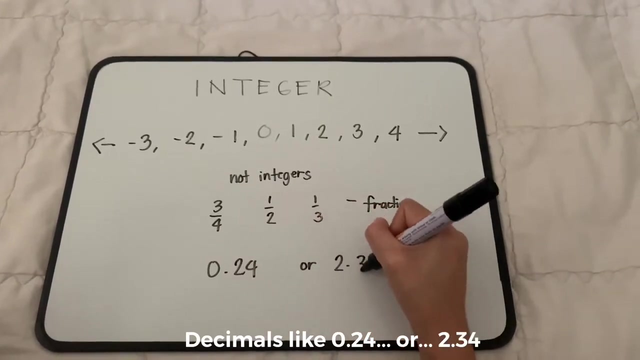 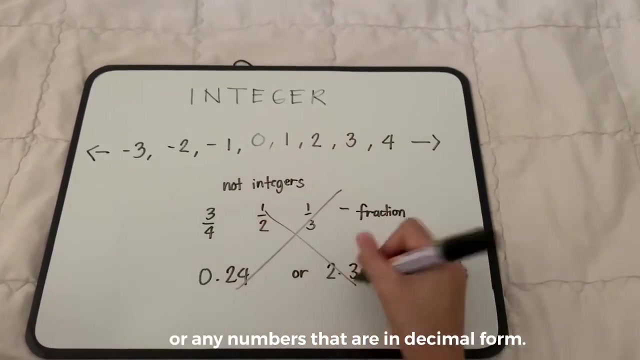 and so on, As long as it's a whole number. So what are those numbers that considered non-integers? Those are fractional numbers, such as three-fourth, half, one-third or any fractional numbers are not considered integers. Decimals like 0.24 or 2.34 are examples of non integers, or any numbers that are in. 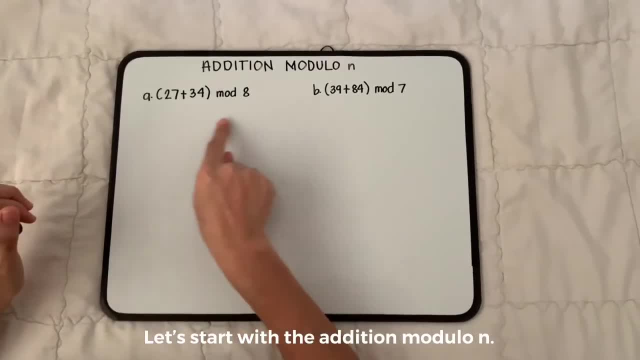 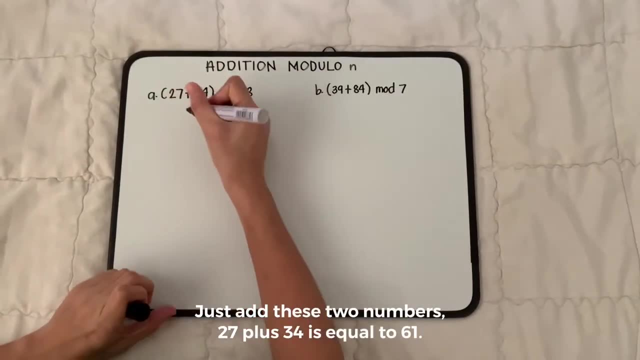 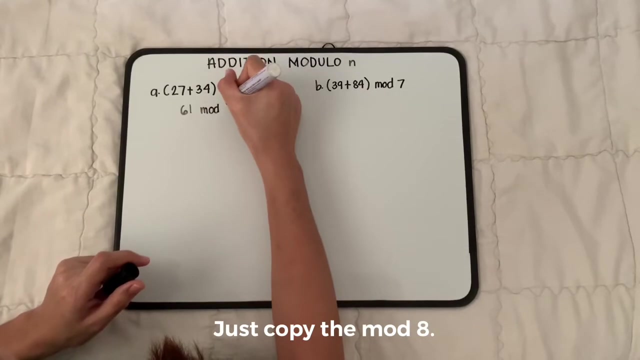 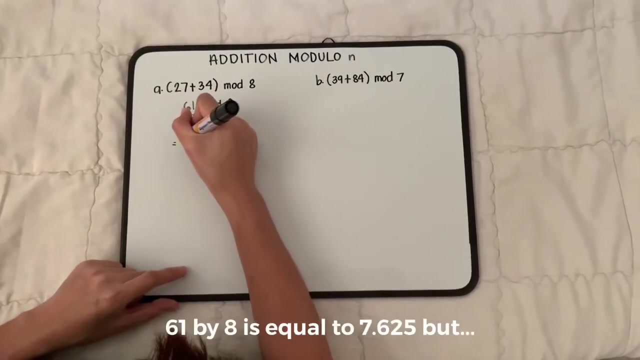 decimal form. Let's start with the addition modulo n. We have two items here. Let's start with the first item. Just add these two numbers: 27 plus 34 is equal to 61.. Just copy the mod 8 and then divide 61 by 8.. 61 by 8 is equal to 7.625. 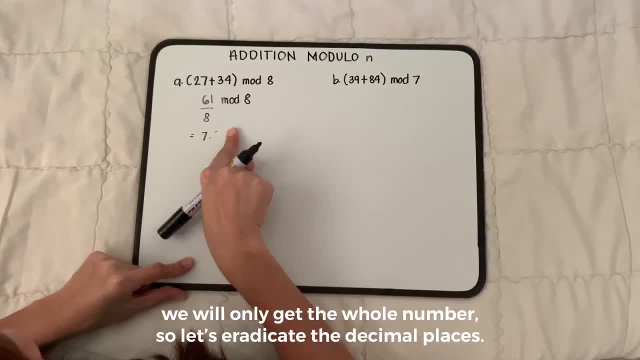 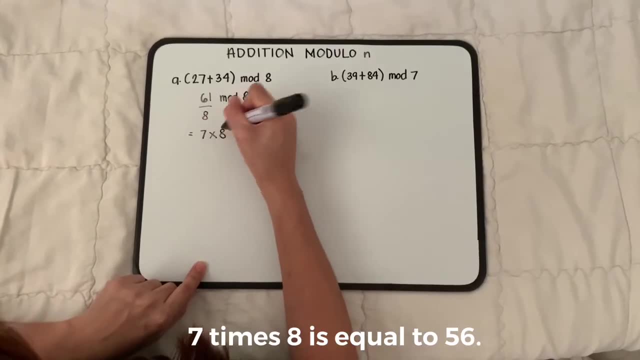 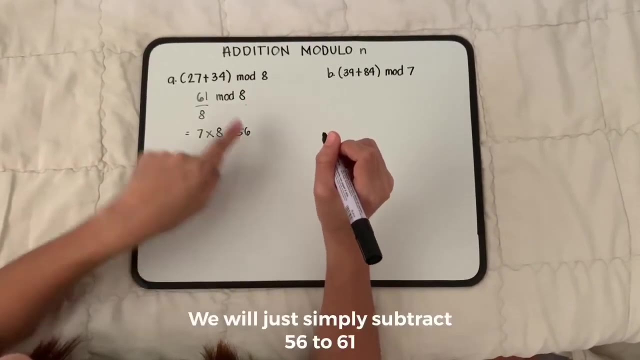 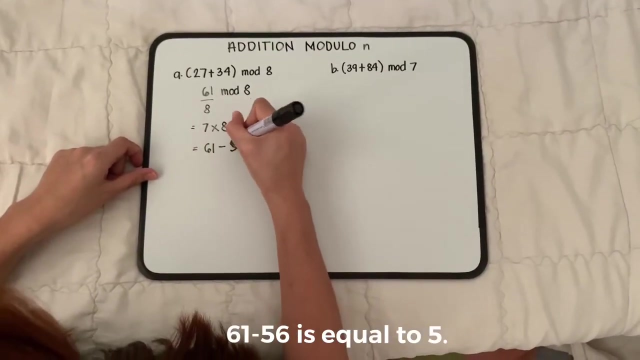 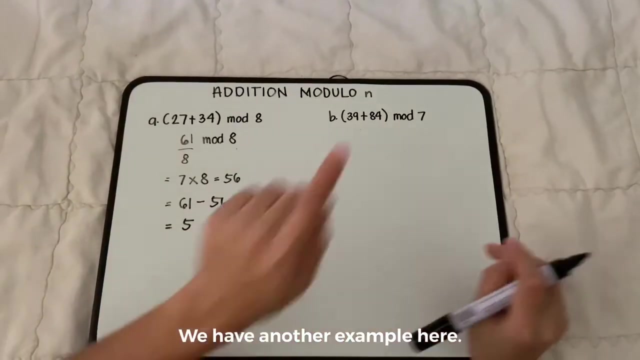 but we will only get the whole number, so let's eradicate the decimal numbers here. 7 times 8 is equal to 56. So we will just simply subtract 56 to 61. So 61 minus 56 is equal to 5.. We have another example here. So 39 plus 84 is equal to. 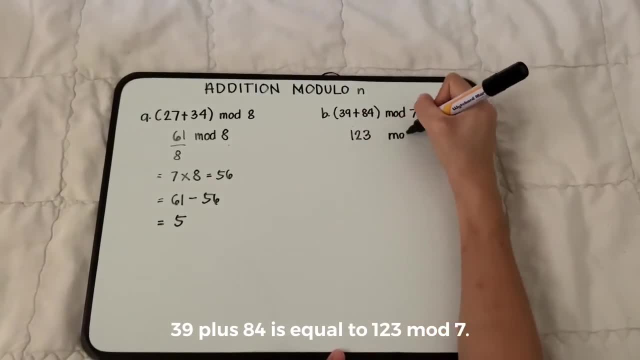 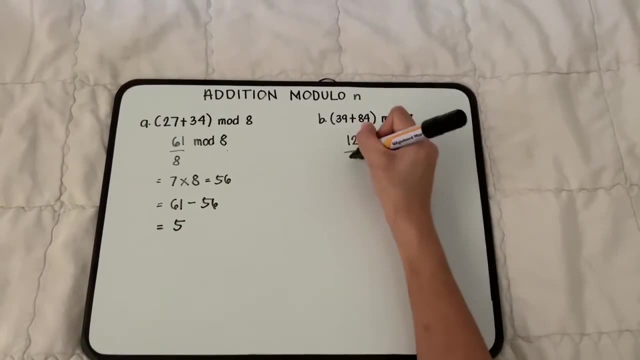 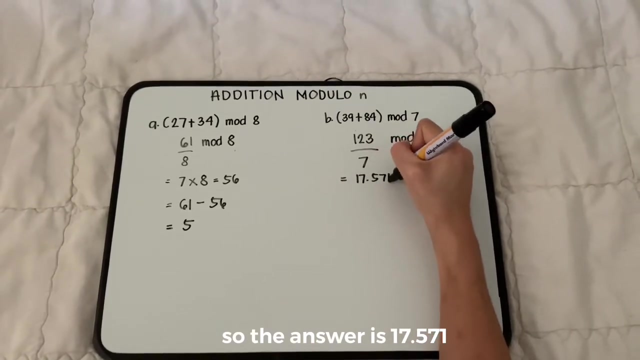 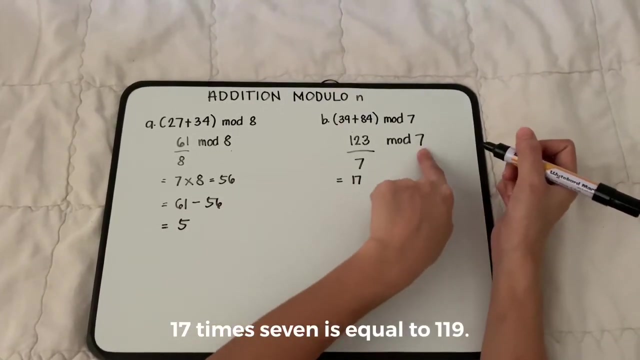 123 mod 7.. Then just simply divide 123 by 7.. So the answer is 17.571, and again we only need the 17. So 17 times 7 is equal to 123 mod 7.. Then just simply divide 123 by 7.. So the answer is 17.571, and again we only need the 17. So 17 times 7 is equal to. 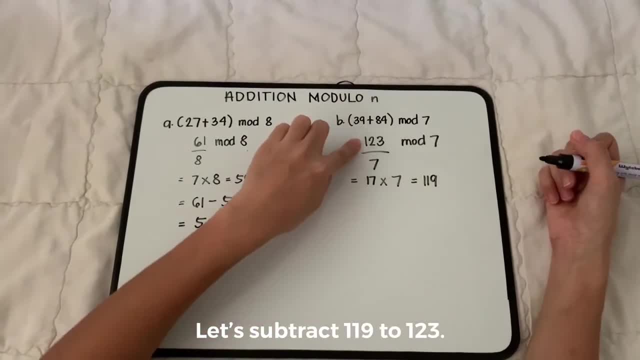 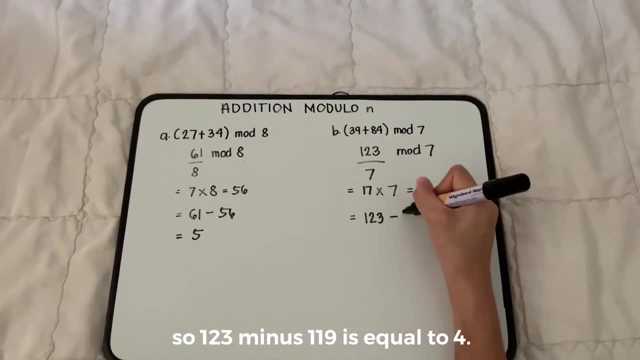 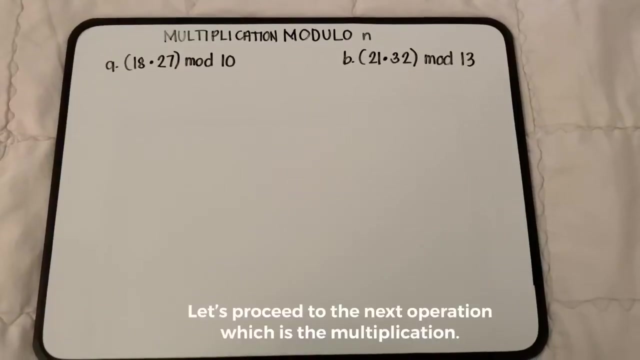 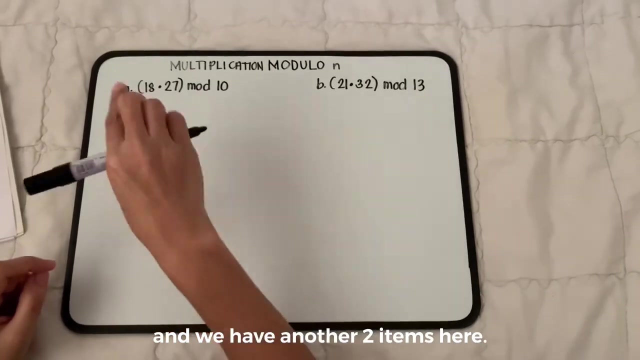 119.. And again, let's subtract 119 to 123.. So 123 minus 119 is equal to 4.. Let's proceed to the next operation, which is the multiplication. and we have another two items here. Let's start. So 18 times 7: since it is a multiplication, we will multiply it. 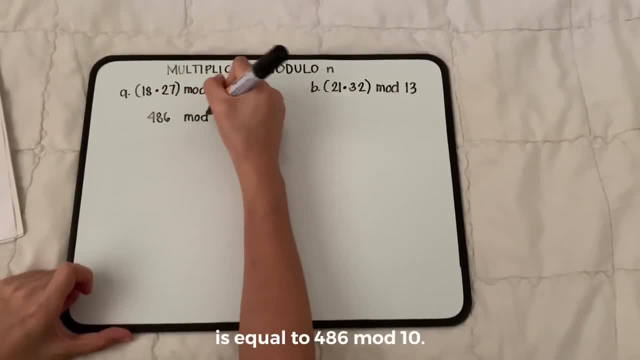 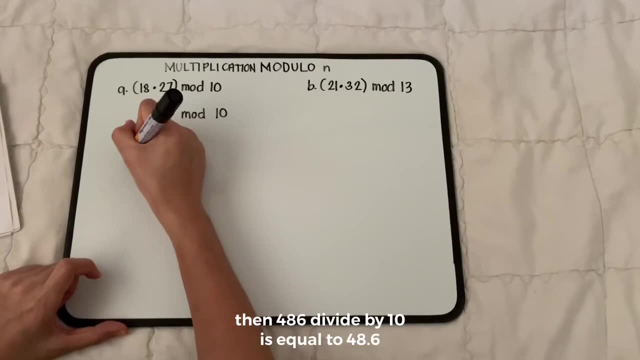 We will multiply the two numbers is equal to 486 modular, then 486 divided by 10 is, and then 436 is equal to 48.6, and the rule is: erase the decimal places and then 48 times. This time is not the one we celebrate, but this is around the여 or зам 0 for사ing. 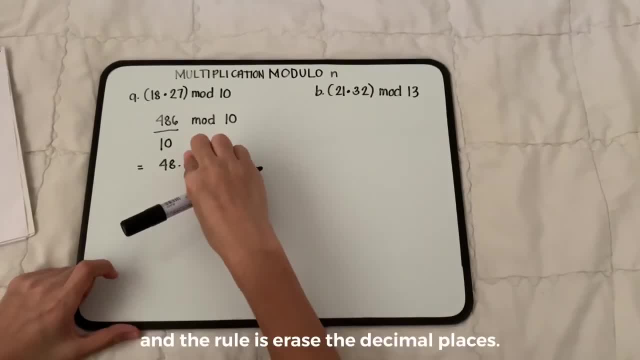 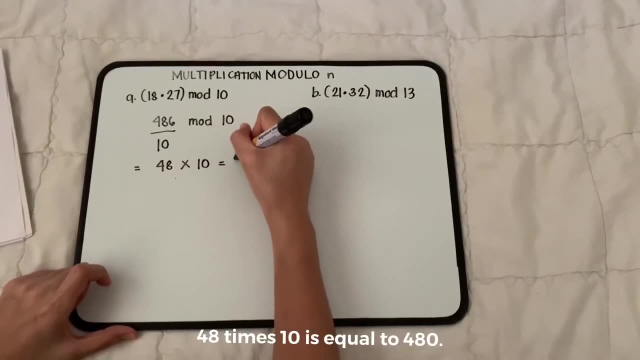 48.6, and the rule is: erase the decimal places and then 48 times 10 is equal to 480.. So 480 subtract one number, and so 48 is equal to. and then, just like last time, If you have newuler, you have to subtract 4 from 20, so 1.. 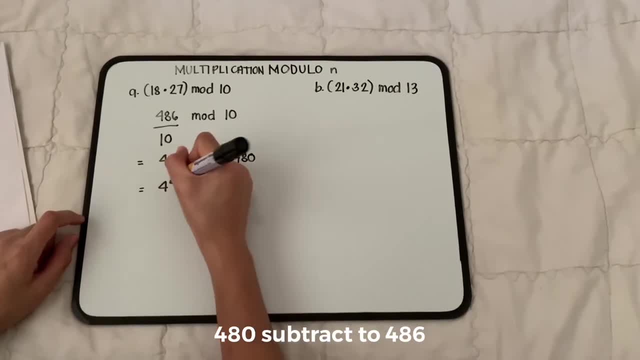 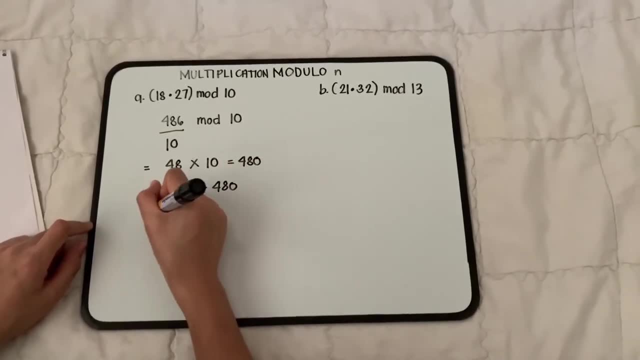 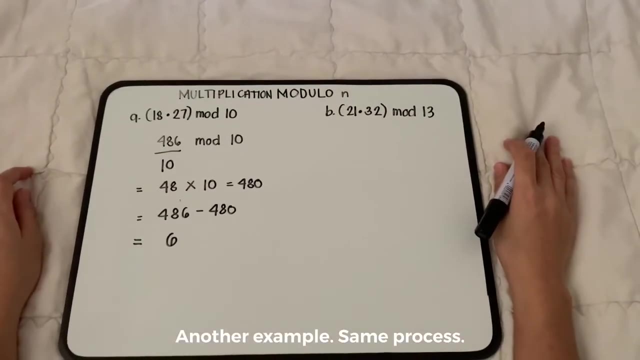 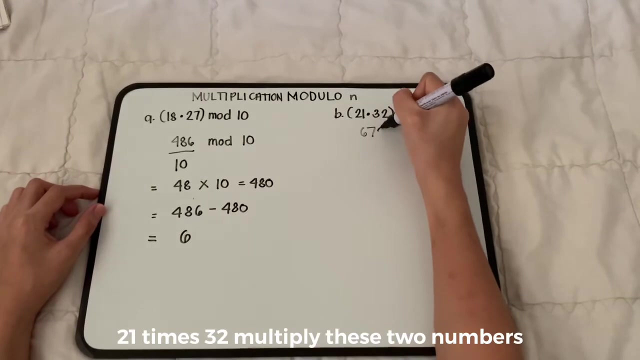 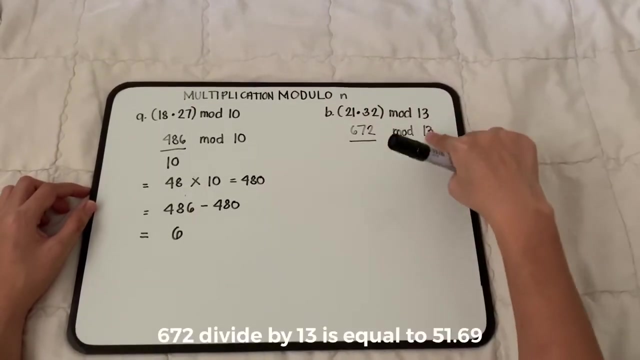 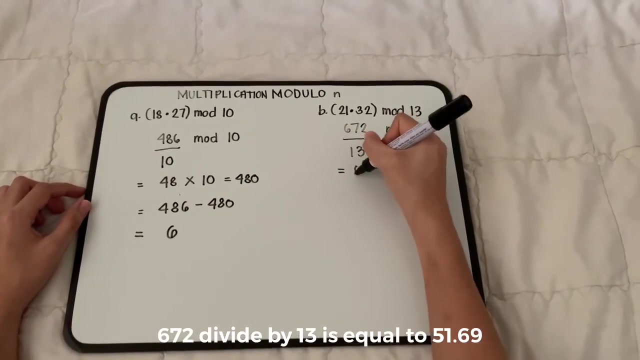 Then, just like last time, If you have newuler, you have to subtract 1 from 20, so 1.. 480 subtract to 486, 486 minus 480 is equal to 6.. Another example: same process: 21 times 32, multiply these two numbers is equal to 672 mod 13, and 672 divided by 13 is equal to 51.69.. 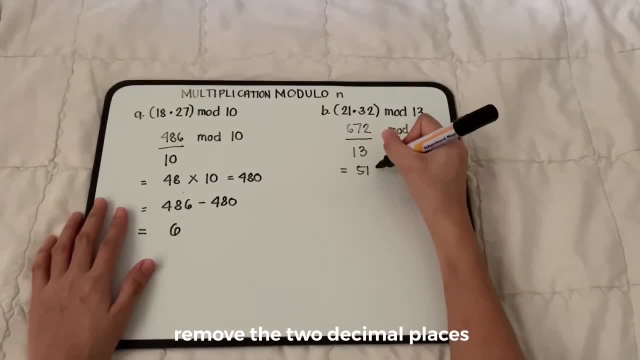 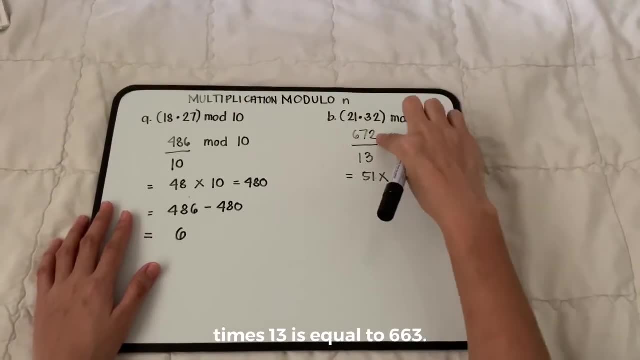 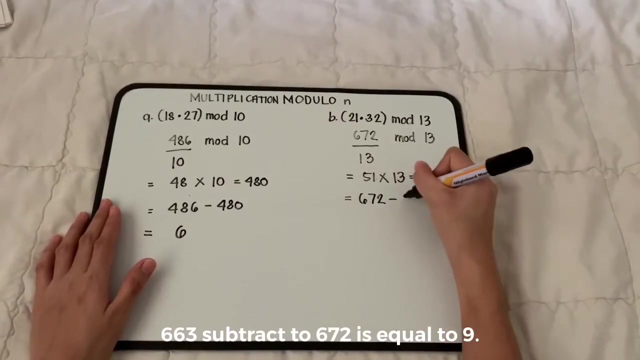 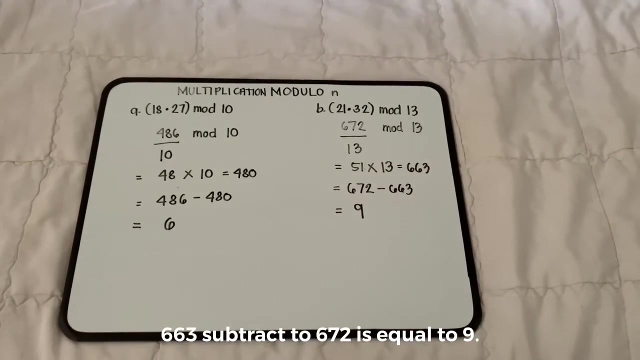 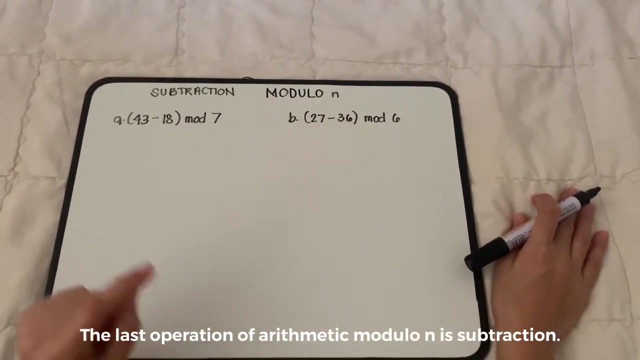 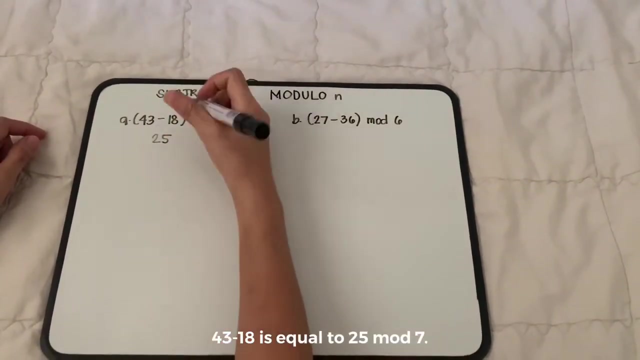 Remove the two decimal places Times 13 is equal to 663.. 663 subtract to 672 is equal to 9.. The last operation of modulo n is subtraction. We have another two examples. So 43 minus 18 is equal to 25 mod 7.. 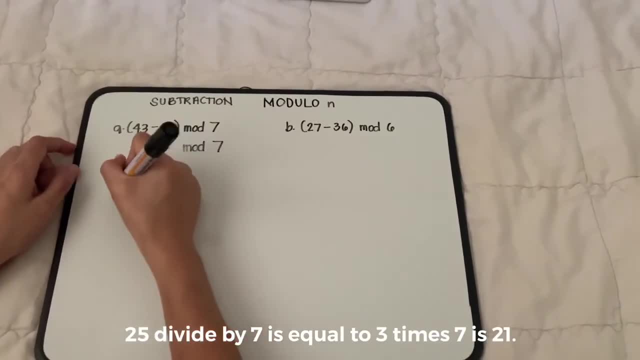 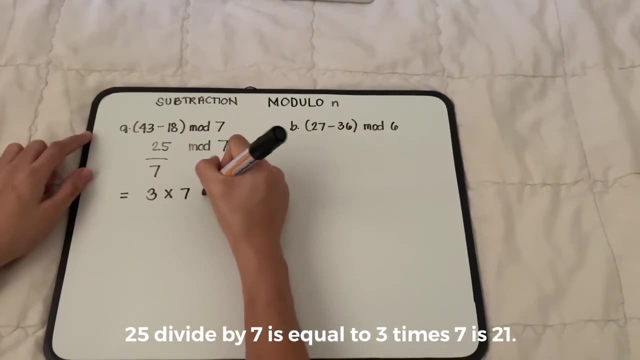 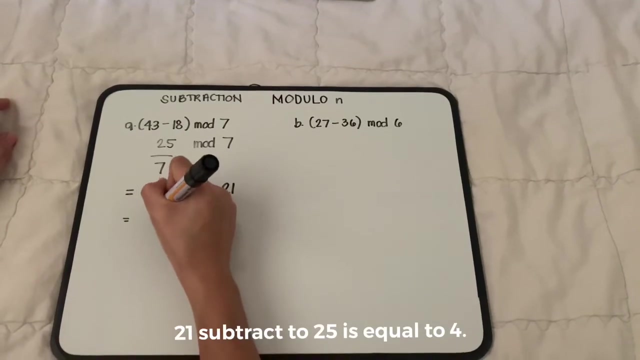 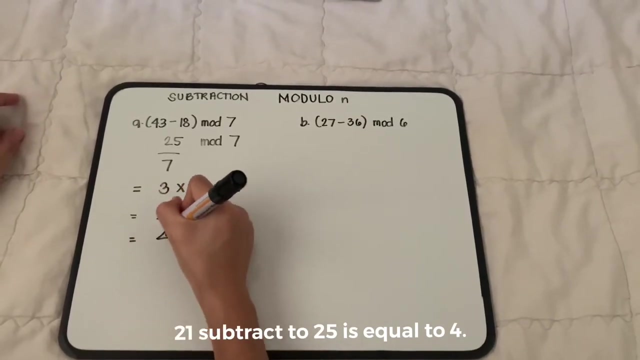 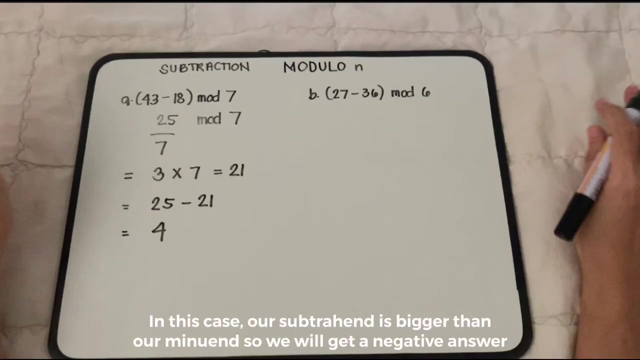 25 divided by 7 is equal to 3.. Since it's a whole number, 3 times 7 is equal to 21.. 21 subtract to 25.. 3 times 7 is equal to 4.. In this case, our subtrahend is bigger than our minuend. 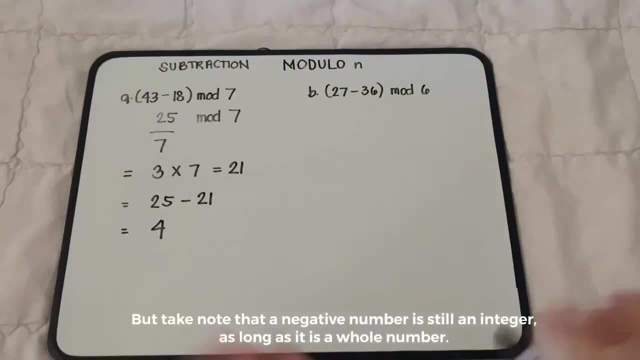 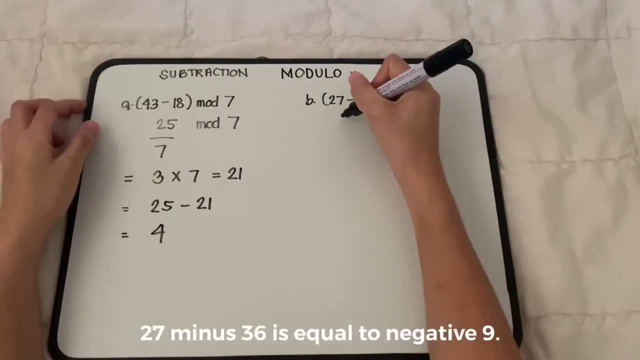 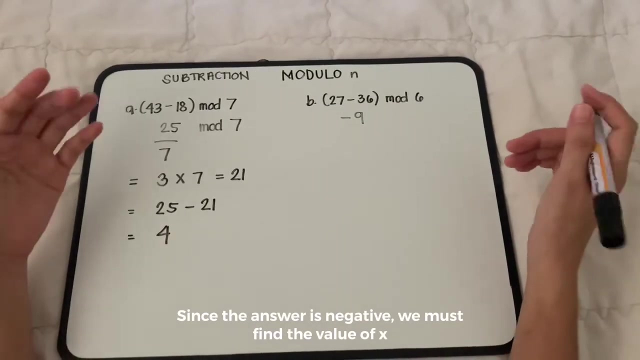 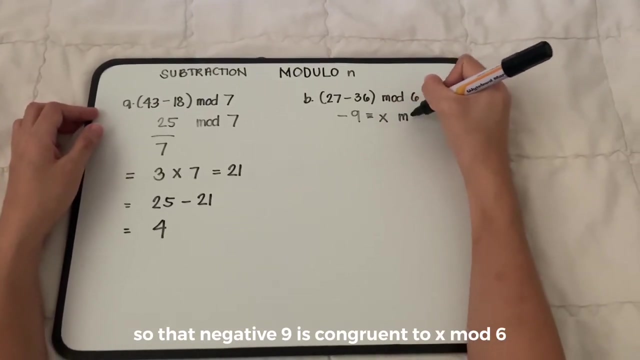 So we will get a negative answer. But take note that a negative answer is still an integer as long as it's a whole number. 27 minus 36 is equal to negative 9.. Since the result is negative, we must find the value of x so that negative 9 is congruent to x mod 6.. 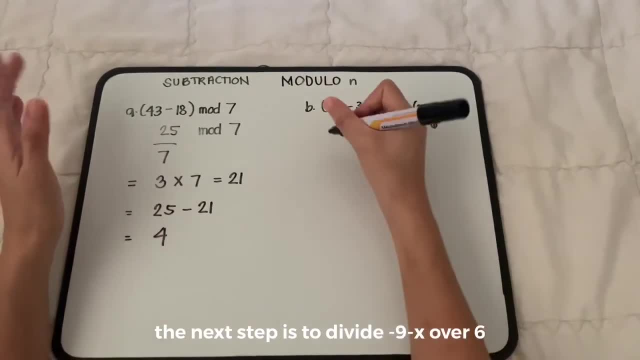 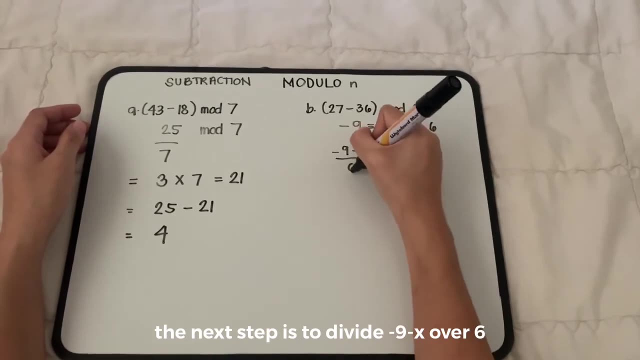 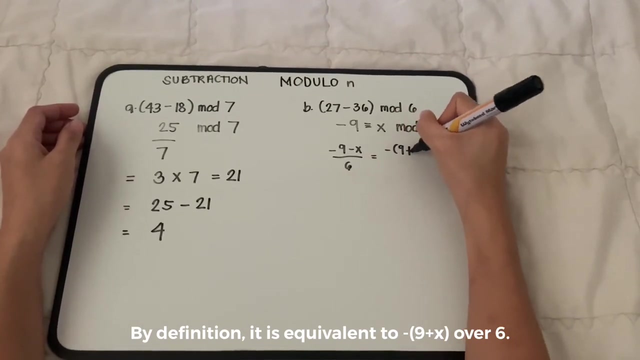 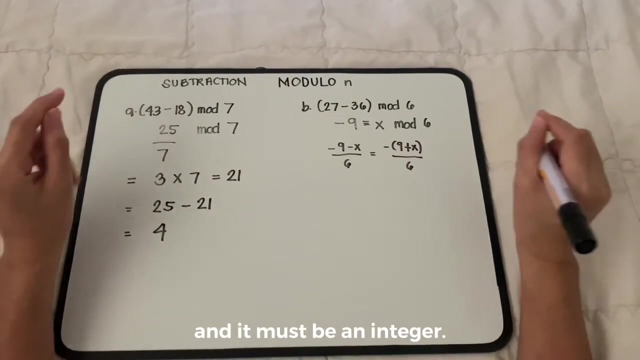 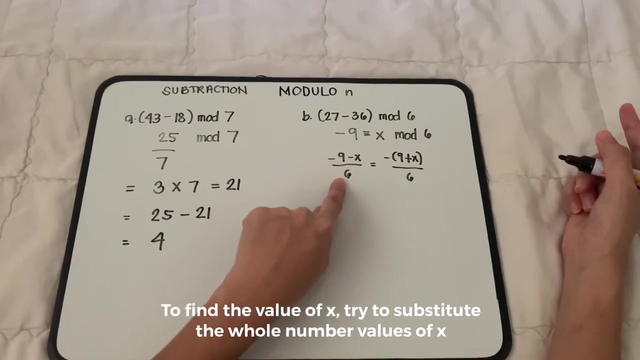 The next step is to divide the negative 9 minus x over 6.. By definition it is equivalent to negative 9 plus x. It must be an integer To find the value of x. try to substitute the whole number values of x less than 6.. 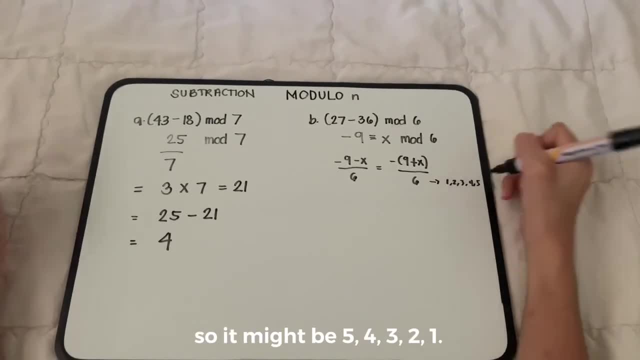 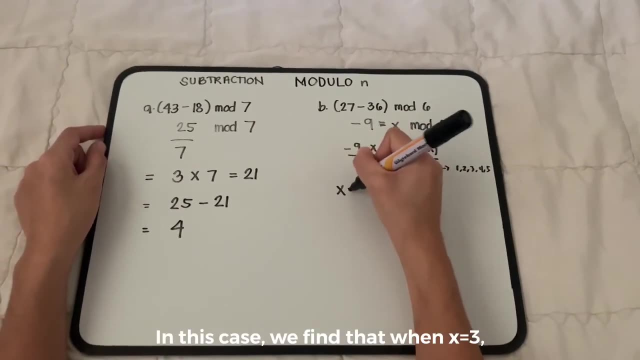 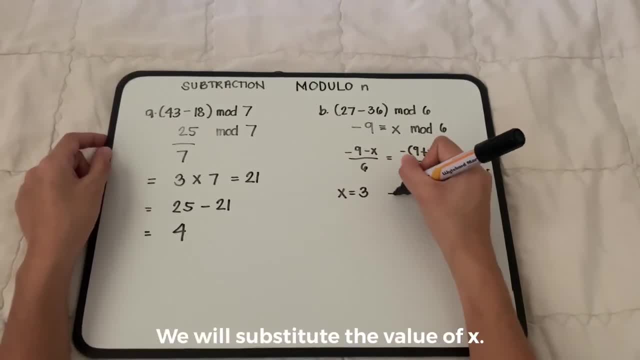 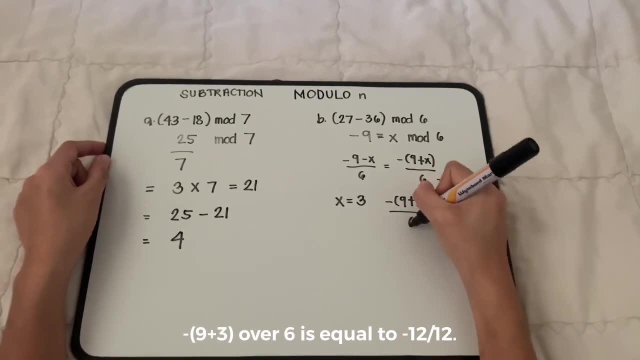 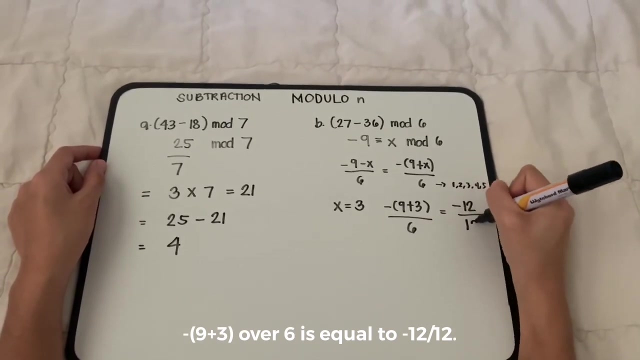 we find that when x is equal to 3,, we will substitute the value of x. negative 9 plus 3 over 6 is equal to negative 12 over 12, and when we divide negative 12 by 12, is equal to negative 1.. 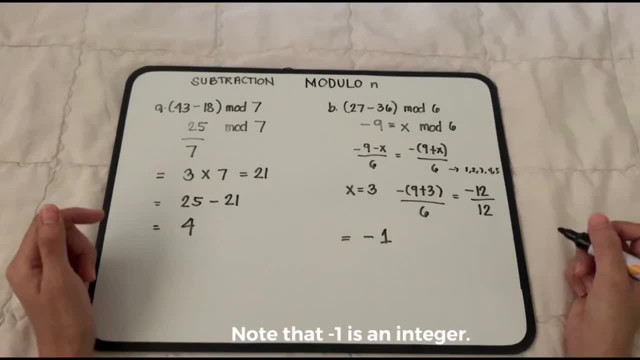 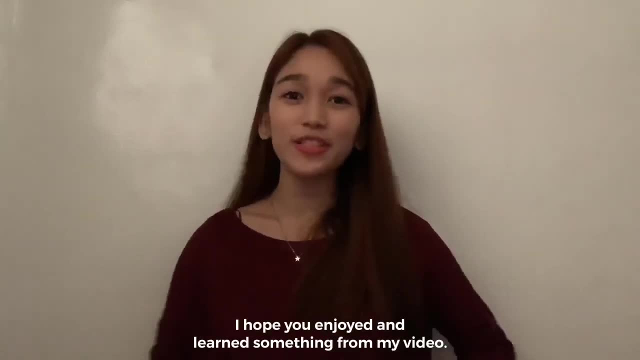 Note that negative 1 is an integer. So that's the 3 arithmetic options operations of model n and I hope you enjoyed and learned something from my video and I hope you can use that in the future.